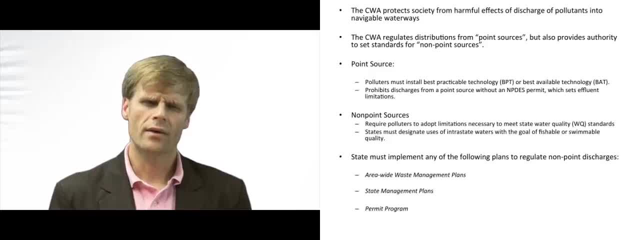 the non-point source polluters. Think of spraying crops and the runoff ultimately ends into navigable water waves. Again, this is a polluter, but it's a non-point source. To start with, what does it require for point source polluters? Well, it uses a scheme of best available technology. 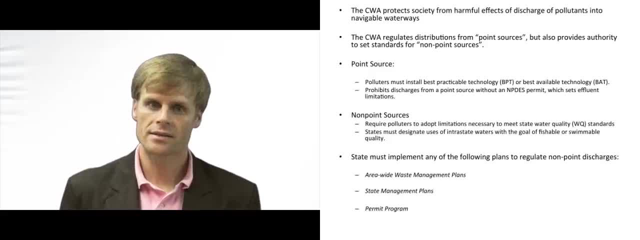 and best feasible or best practical technology to prevent pollution or the discharge of pollutants into navigable water waves. And it has a permit scheme that sets affluent standards that, in the event you are going to discharge from a point source, you have to get a permit and 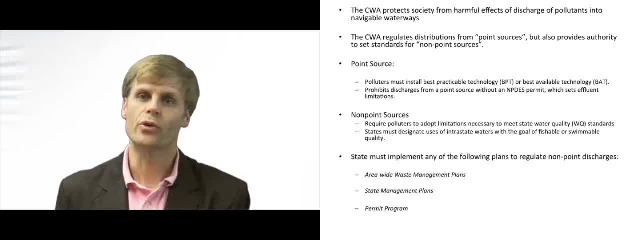 meet these standards or criteria for the amount or percentage of pollutant that you can discharge into the water waves. Okay, and for the non-point source, while it doesn't regulate it directly, What it does is it requires states to set certain water quality standards, and these non-point. 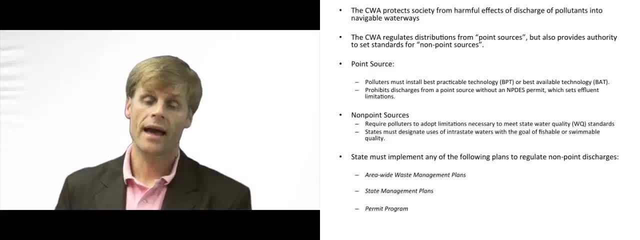 source dischargers may have to limit their activity to meet these standards. So what it allows is the state to adopt any number of plans. The 3 types of plan is a water management plan, which is a прибro saatation management plan, that is, an respecting list, or a local. 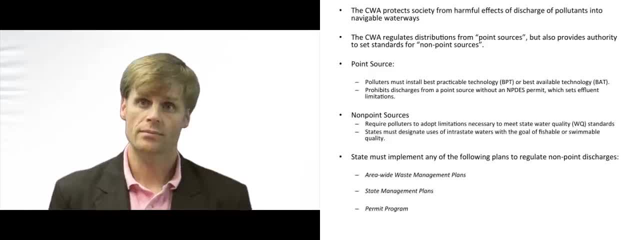 an approach where you treat water to arrive at the appropriate percentage of materials or pollutants in the waterways. You can have just a water management plan where it uses all sorts of criteria for dischargers with the ultimate goal of meeting these water quality standards, or you could have a permit. 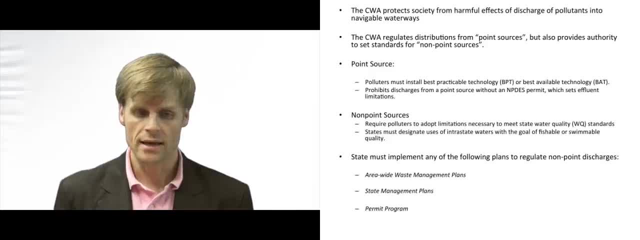 system similar to what the federal government uses in a number of instances. If the state does this, it has to set certain standards for the water. it has to designate whatever standard or quality of water you're trying to get to- whether it's swimmable, fishable. 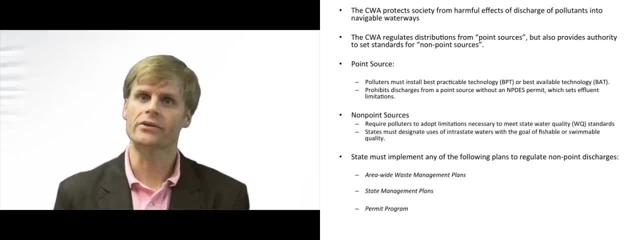 whatever, and it has to set certain particular standards in the water. to meet this standard, It has to implement or enforce some sort of plan or regime to make non-point swimmable source dischargers into the waterway meet these standards. Like I said, it could be through any number of plans.